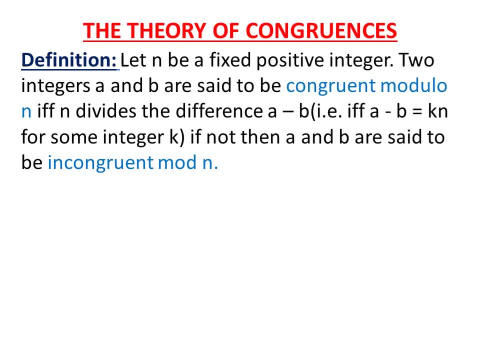 if n divides the difference a-b, That is by definition of divisibility. if we can find some integer k such that a-b can be written as k into n, then we say that a and b are congruent modulo n. or we can say a is congruent to b mod n. So if n does not divides the difference, 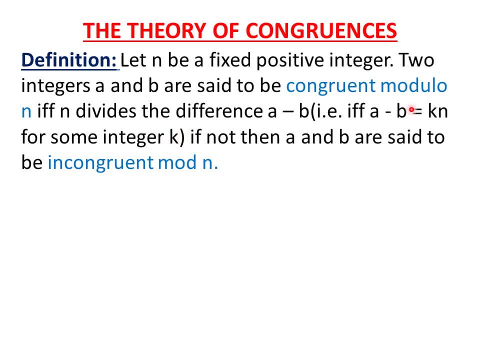 a-b, that is, if we cannot find some integer k such that a-b equals k into n, then a and b are said to be incongruent. So what is incongruent modulo n, That is a, is incongruent to b, mod n. So the notation 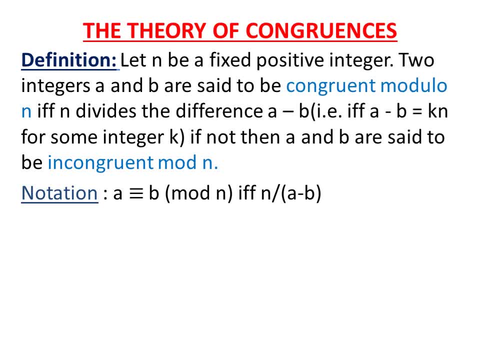 used to denote it is as follows: a is congruent to b mod n is denoted by this notation and this happens if, and only if, n divides a-b and a is incongruent to b modulo n notation is this: and it happens if n does not divide a-b, For example. here we can see the difference. 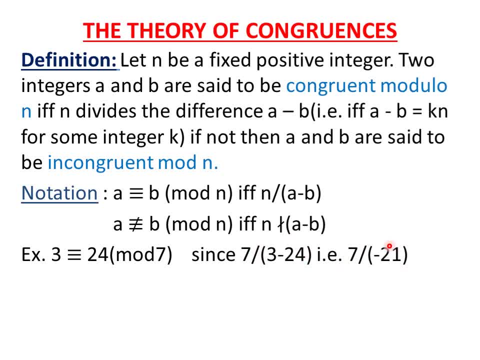 a-b is 3 minus 24, which is minus 21, and clearly 7 divides minus 21. therefore we can say 3 is congruent to 24 mod 7.. But in next example, 25 minus 12 is 13 and 7 does not divide 13. therefore here 25 is. 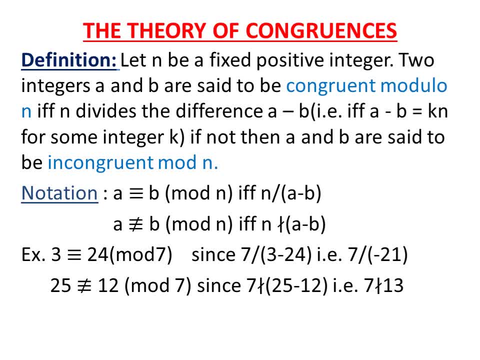 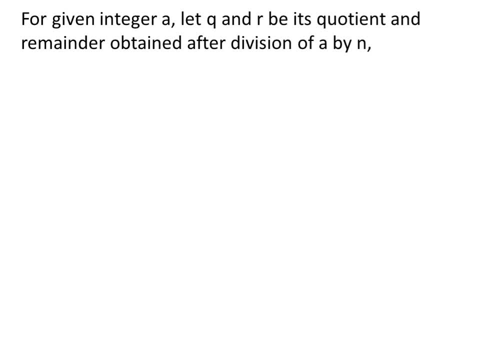 not incongruent to 12 mod 7.. So these are the examples For: given integer a, let q and r be its quotient and remainder obtained after division of a by n. Thus, by using division algorithm, we can write a equals qn plus r, with the restriction on remainder r as remainder can. 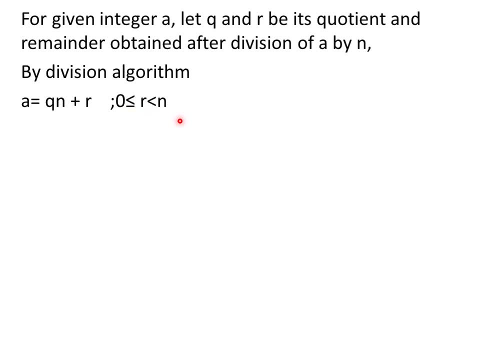 be 0 or greater than 0, but strictly less than divisor, that is n. So this statement can be written as this: that is, a minus r equals q into n. As q is integer, this implies, by definition of divisibility, n divides a minus r. So by using definition of congruences, I can write: a is: 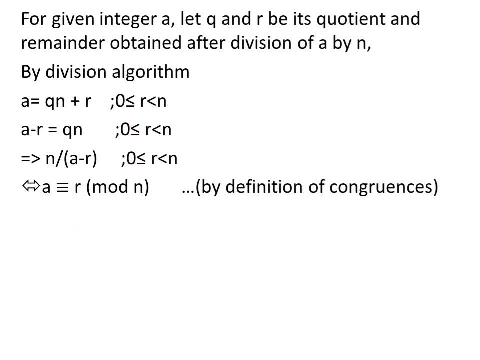 congruent to r mod n. with this restriction on remainder r, Because there are n choices for r, we see that every integer is congruent, modulo n, to exactly one of the values 0,, 1,, 2, up to so on n minus 1.. Because of this constraint, if we divide any integer by n, 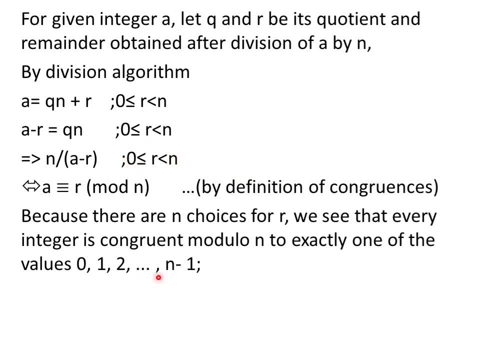 we get n minus 1.. So by using definition of congruences I can write: a is congruent to r mod n, then there are this n choices for the remainder r. In particular, if I will say a is congruent to 0 mod n, then this implies n divides a. or if I will say n divides a, then this implies a is congruent. 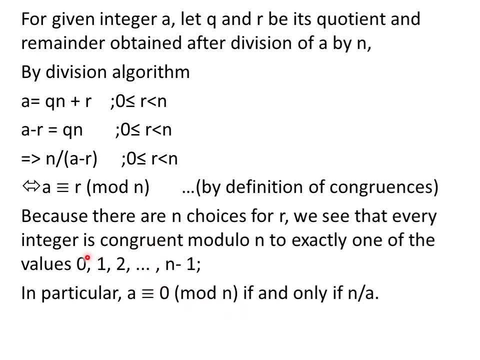 to 0 mod n. So whatever the remainder we are getting, all are positive and they are the least such a integers. So the set of integers 0, 1, 2, up to so on n minus 1 is called as least non-negative residues. 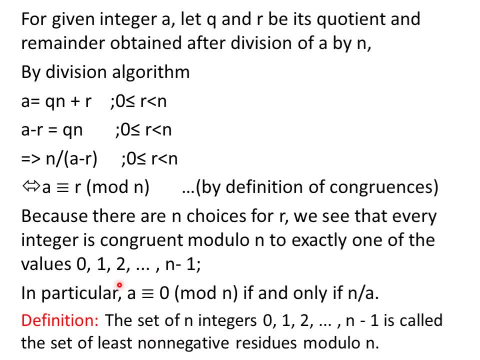 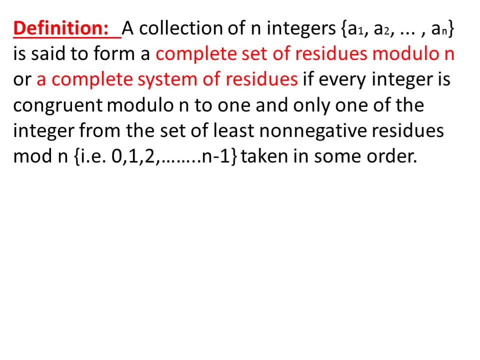 modulo n. So that is this definition of least non-negative residues, modulo n. Let us define one important term from congruences: A collection of n integers, say an a1, a2, up to so on, a n is said to form a complete set of residues, modulo n, or a complete set of residues, modulo n. 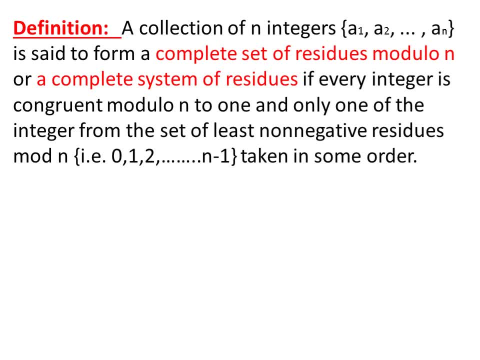 Next step is n based system of residues. if every integer is congruent, modulo n to one and only one of the integers from the set of least non-negative residues, mod n, that is this set, and this is taken in some order. This definition says that if I will divide, 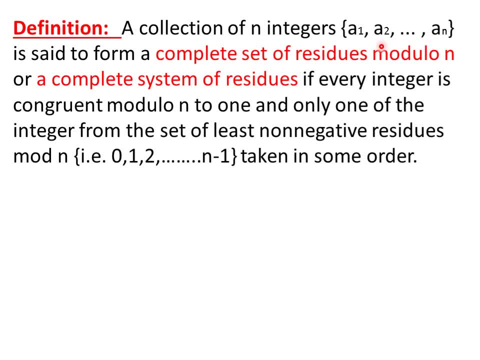 this, integers a1, a2, upto so on, by n, then I must get the remainder from this set or from here, So I go for 0. And there are only 2 integers are there? so I divide them by n. by n간코 1, n is said to. 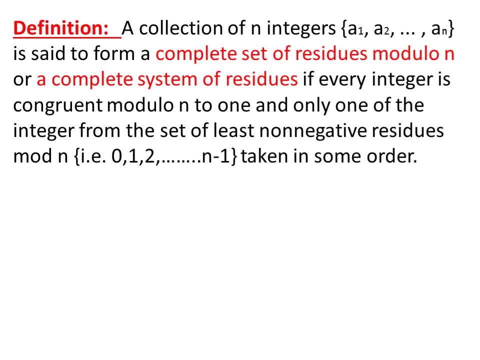 no two integers should get the same remainder. so if i will get such a type of set which satisfies these two condition, then i will say this set forms a complete set of residues, mod n or complete system of residues, for example. let us check whether this set forms a complete. 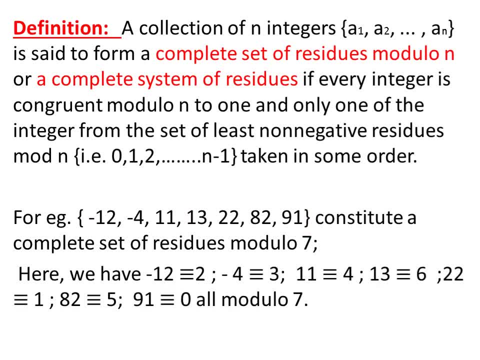 set of residues, mod 7 or not. if i will divide this integers by 7, then i will remainder. i will get remainders as follows: that is, for minus 12, 2 for minus 4, 3 for 11, 4 for 13: 6. 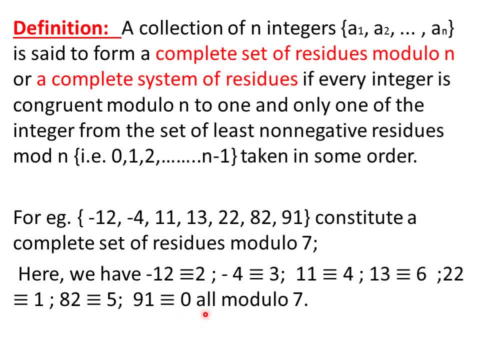 for 20 to 1, for 80 to 5 and for 91: 0. so here i can see. all of these remainders are from the set 0, 1, 2, up to so on 6, which is the set of least non-negative residues. modulo n: right. 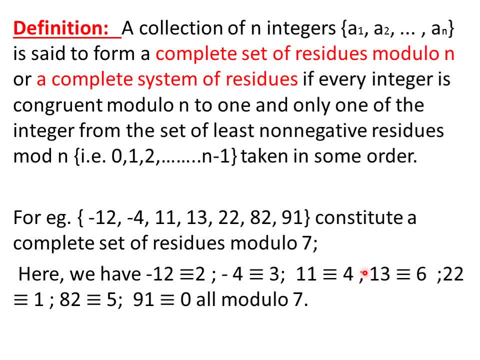 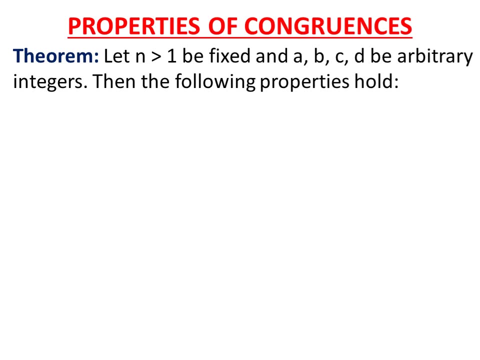 and none of the two integers from the set got the same remainder. so i can say that this whole set of integers forms a complete set of residues, mod 7. so this is example for it. let us see some properties of congruences. so for this, let n greater than 1 be a fixed. 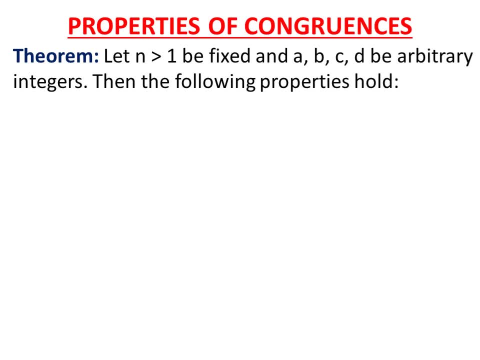 integer, and a, b, c, d are some arbitrary integers. then for this, following properties holds first: one: a is congruent to a, mod n. this property is called as reflexivity, which says any integer is congruent to itself, mod n. next let's discuss the set of non-negative residues, mod 7. so this set of integers is: 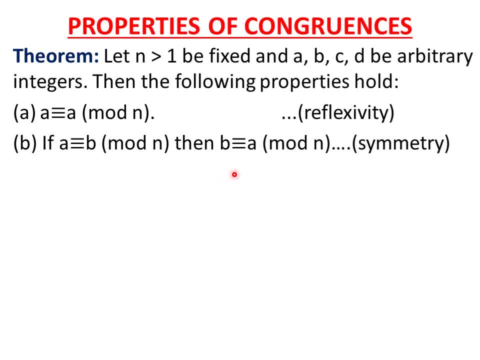 the set of non-negative residues, mod 6, which is the set of non-negative residues, mod 8, which one? if a is congruent to b- mod n- then b is congruent to a- mod n, so this property is called as symmetry. next one: if a is congruent to b- mod n- and if b is congruent to c- mod n- then 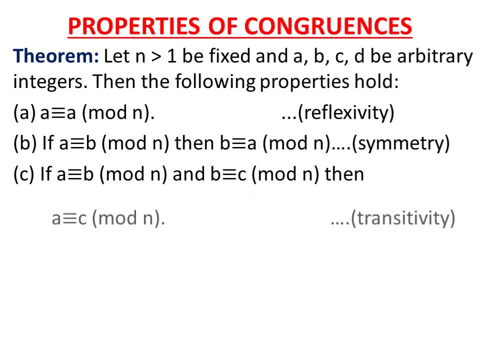 this integer: a is congruent to c mod n. that is this. this property is called as transitivity. next one: if a is congruent to b mod n and if c is congruent to d mod n, then i can say: a plus c is congruent to b plus d mod n, and a into c is congruent to b into d mod n. that is this. 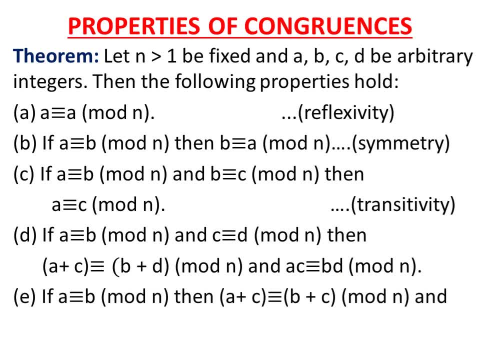 next, if i have a is congruent to b mod n, then i can add any derivative positive or negative integers on both sides so that i will get a plus c congruent to b plus c mod n and i can multiply by some integer on both side, that is ac congruent to bc mod n. 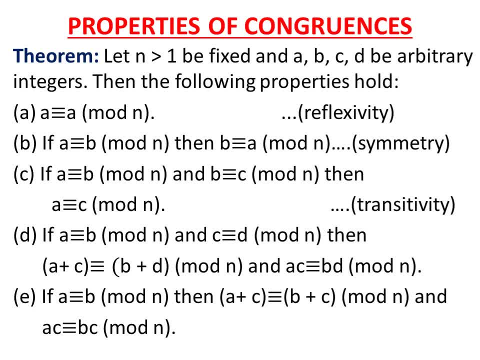 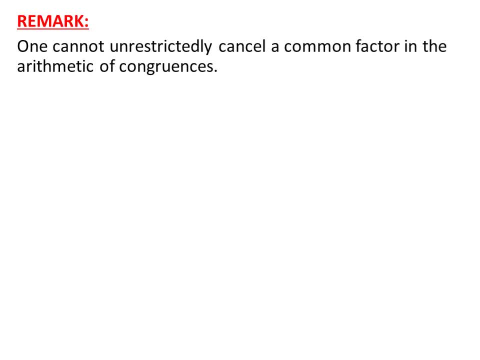 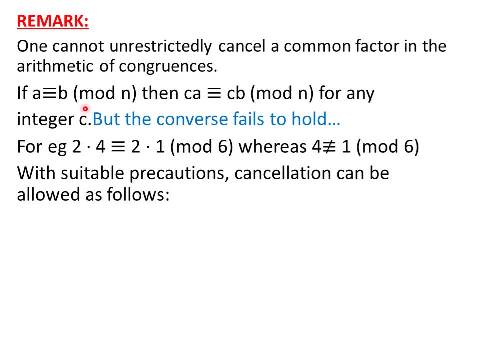 so these are the all properties of congruences. note that one cannot unrestrictedly cancel a common factor in arithmetic of congruences. in properties of congruences we have seen: if a is congruent to b mod n, then ca is congruent to cb mod n for any integer c, that is for this. 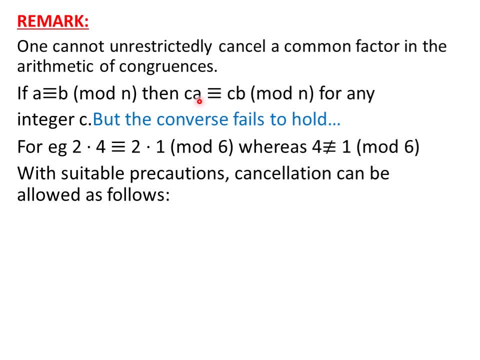 congruence. we can multiply by some integer c and we can say this statement, but converse of this statement fails to hold. that is, if we have this congruent ca, congruent to cb mod n, then we can not cancel this common factor c on both side. so if we'll cancel this common factor c, then we'll 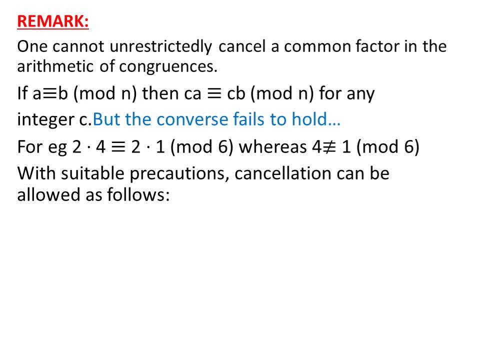 get a congruent to b mod n, which is not always true. for example, here we can see: 2 into 4 is 8, 2 into 1 is 2 and 8 minus 2 is 6 and 6 divide 6. therefore this congruence holds, but if we'll 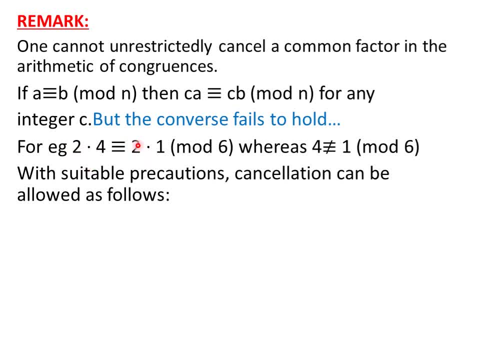 cancel out this common factor 2, then we'll get 4 congruent to 1 mod 6, which is not true, because 4 minus 1 is 3 and 6 does not divide 3. so the converse of this statement is failed here right. therefore, one cannot cancel out common factor unrestrictedly. 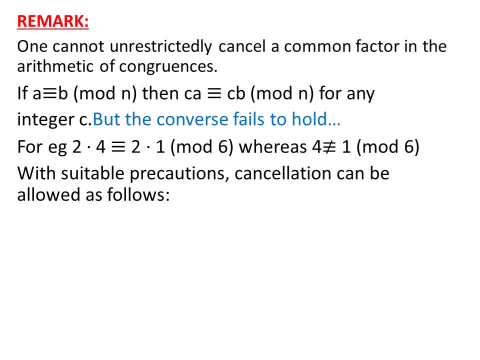 so if we'll take some precautions while cancellation, then cancel out this common factor 2, then we'll get 4 congruent to 1 mod 6, which is not true. so cancellation is allowed. so which can be stated by following theorem. that theorem says: if c, a is congruent to c, b mod n, then a is congruent to b mod n by d, where d is a gcd of. 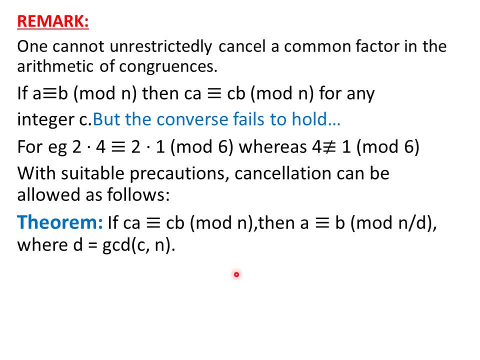 c and n. okay, so by using this theorem, if we have gcd of c and n as 1, then this factor d will be 1.. right, that means this term, the n upon d, that will be just n. so in that case we can say: if we have 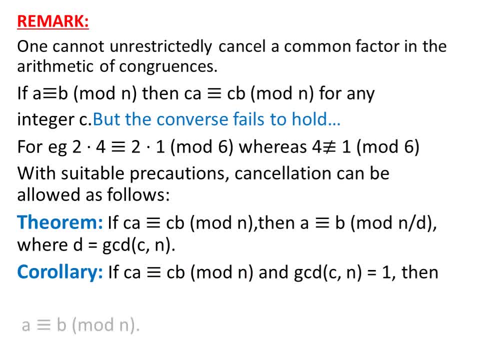 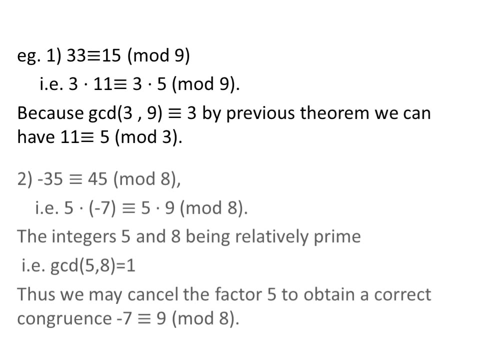 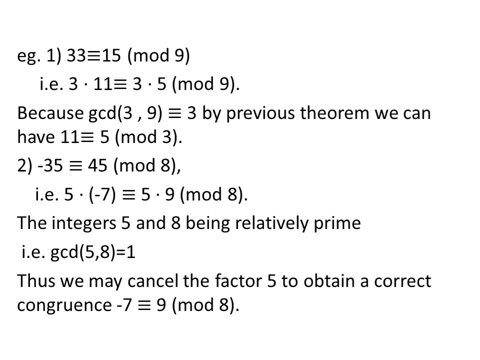 c. a is congruent to c, b mod n. and if gcd of c and n is 1, then this will imply a is congruent to b mod n. so without some precautions we cannot cancel common factor. note this based on previous remark. these are some examples. you can refer this for your better understanding. 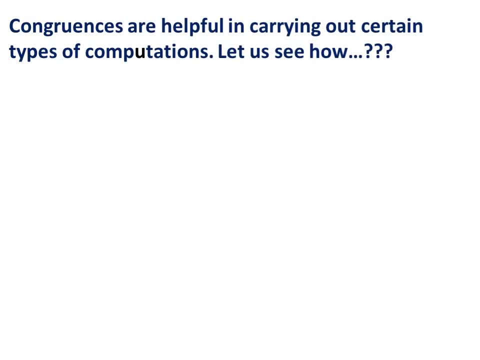 congruences are helpful in carrying out certain type of computations. let us see how, in this example, we want to show that 41 divides 2 raised to 20 minus 1. so to do this, we will start with the term 2 raised to 20, we will divide it by 41 and we will find out its remainder. so to do this, 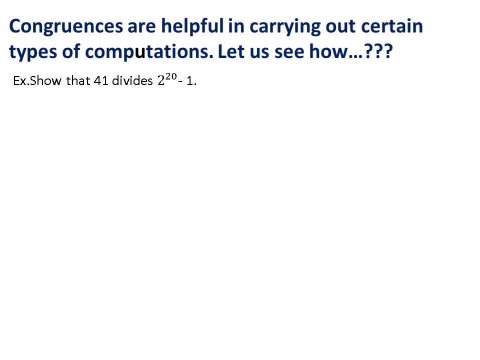 we will use congruence. so let us see how to do it. first of all, we will use congruence to find out the value of the term 2 raised to 20 minus 1. we will compute powers of 2 that are 2 raised to 2, 2 raised to 3, and so on. so, among all these powers, 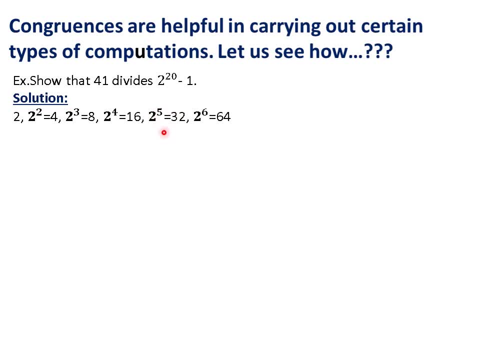 we will select that power for which we are getting closest value to 41. so here we can see: 2 raised to 2 is 4, 2 raised to 3 is 8, 2 raised to 4 is 16, 2 raised to 5 is 32, 2 raised to 6 is 64, and so on. 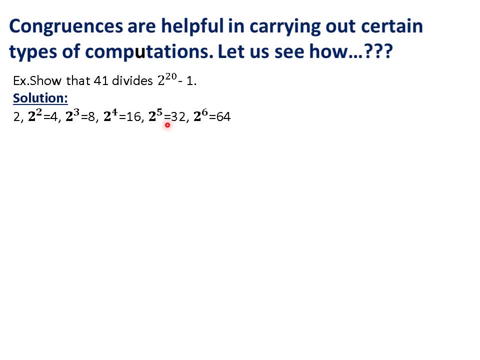 so among these, the closest value to 41 is 2 raised to 2 is 4. 2 raised to 3 is 8. 2 raised to 4 is 16. 1 is 2 raised to 5, which is 32, so we'll consider this. so 2 raised to 5, that is 32 when it is divided. 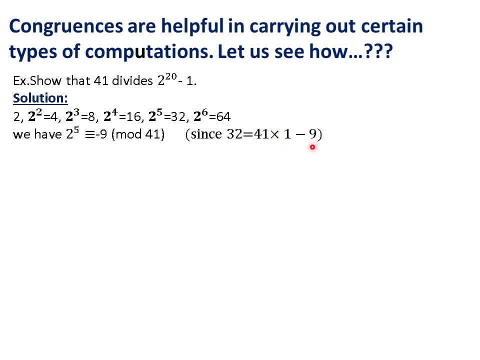 by 41, then we will get remainder minus 9, because we can write 32 as 41 into 1 minus 9. so by division algorithm this is the remainder that is minus 9. so by definition of congruences we can write 2 raised to 5 congruent to minus 9 mod 41.. 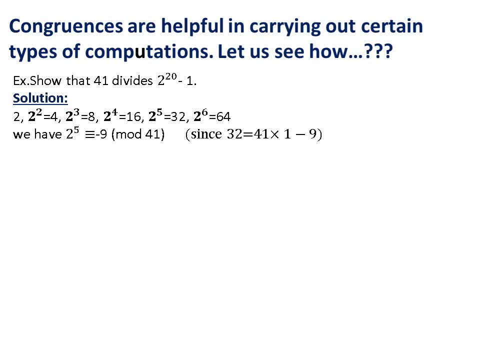 right. we have seen properties of congruences by using it, since here we want the power of 2 as 20 and here we got the congruence for the power 2 raised to 5 right, so to get for 40 to get power. 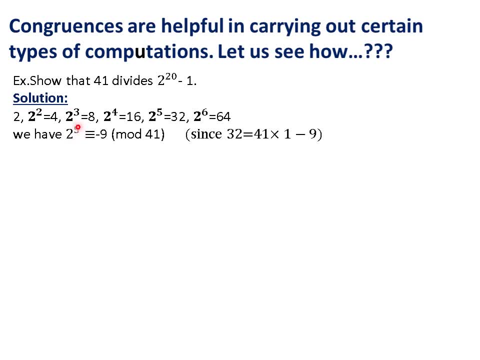 of 2 as 20, we can raise its power to get it as 20. okay, so if a is congruent to 2, raised to 5. if a is congruent to 2, raise to 5. two slide: we will get 3 raised to 1 underscore. so we: 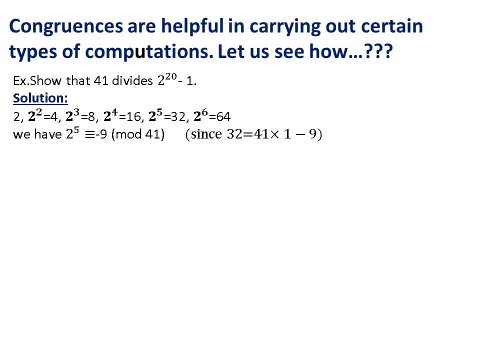 can have square root of 10. alright, now, if it is subscriber, forget the vos moto C. i love this one in bahasa what i have just shown. so let's come to square root of 9. what we got? we have 4 raised to 4 plus 1, which is corresponding to positive integer k, so that is congruent to B mod n. this is congruent to B mod n for some positive integer k. so here what K can be selected? if you select K x 4, then we will get 5 into 4 as twenty con3.0, which is required one. so by raising its power by 4, so that we will get 2, raise to 5, raise to 4 is: 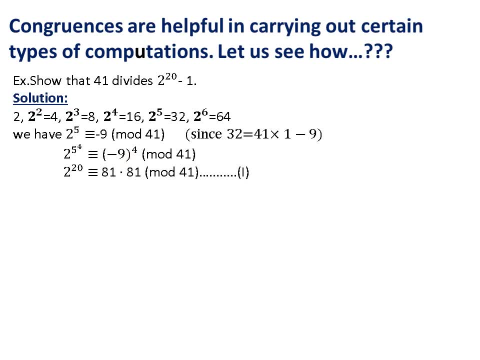 congruent to five. raise to 4, mod 41, but minus 9. raise to 4. consider to 0, which is least. minus 9. raised 4 can be written as 81 into 81, that is, 9 square into 90, 9 square right. so 2 raised to 20 is. 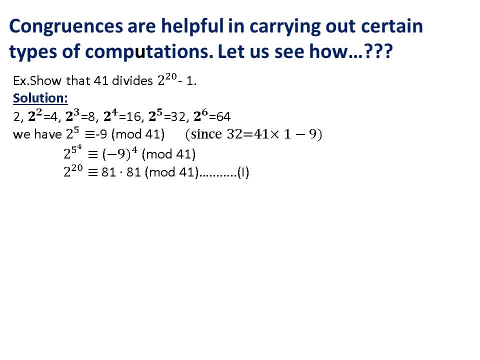 congruent to 81 into 81 mod 41. okay, but we know that when we divide this 81 by 41, they will get remainder as minus 1. you can verify it therefore: 81 into 81, it will be a congruent to minus 1 into minus 1 mod 41. that is just 1 mod 41, right? we have transitivity property of. 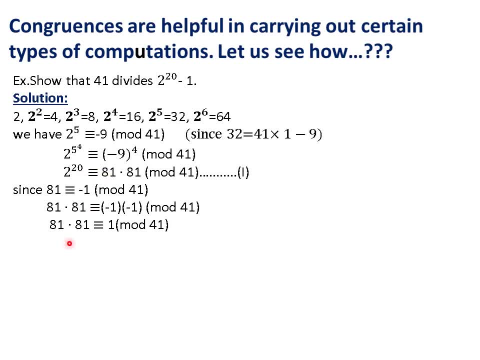 congruences: if a is congruent to b mod n and if b is congruent to c mod n, then a is congruent to c mod n. therefore, we can write by 2 and by using one equation 1 and this equation 2 raised to 20. 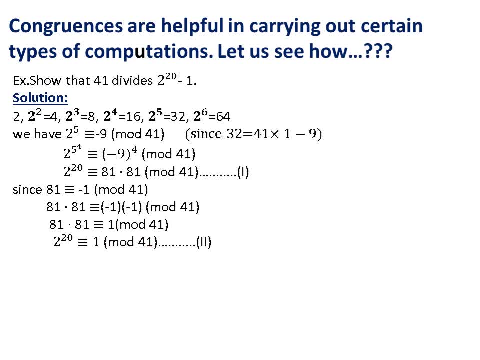 is congruent to 1 mod 41 followed. thus you we got remainder of 2 raised to 20 when it is divided by 41. now consider the term 2 raised to 20 minus 1, that is, that will be 1 minus 1. 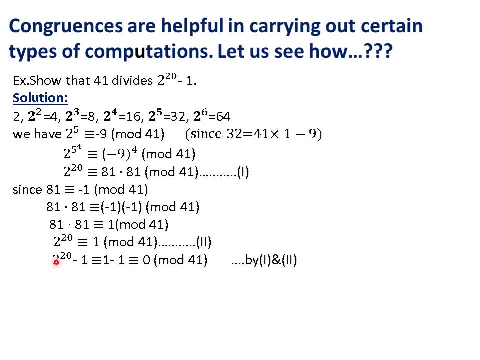 and 1 minus 1 is 0. therefore, 2 raised to 20 minus 1 is congruent to 0 mod 41. that means when we are dividing this term by 41, we are getting remainder as 0 and this implies 41divided 2 raised to 20 minus 1. hence the proof ok. 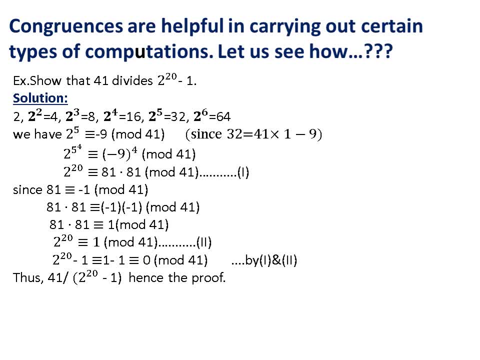 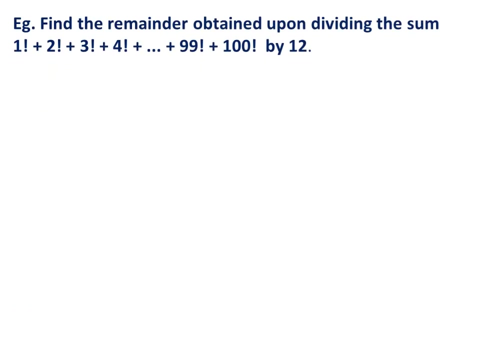 so in this way we can use congruence to solve such a type of examples. so these are some examples for practice. you can solve it. this is one more type of Example which can be solved by using congruences, which can be solved by using congruences. in this example we can solve congruence. user can make such a proof check. 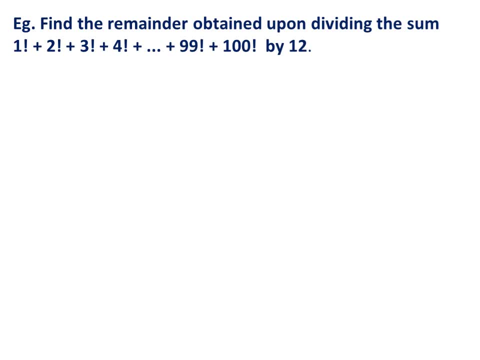 we want to find remainder obtained upon dividing the sum 1 factorial plus 2 factorial plus 3 factorial, up to so on, plus 100 factorial by 12. so for doing this we can use congruences, since we have 4 factorial as 24 and as 12 divides 24, therefore its remainder is 0 when 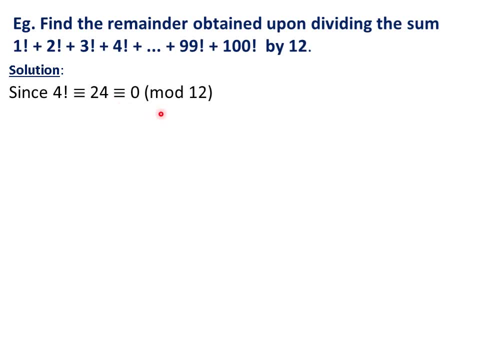 it is divided by 12, so 24 is congruent to 0 mod 12 right. so for all the integers which are greater than or equals to 4, the k factorial contains the factor 4 factorial right. so for integers k greater than or equals to 4, we will have 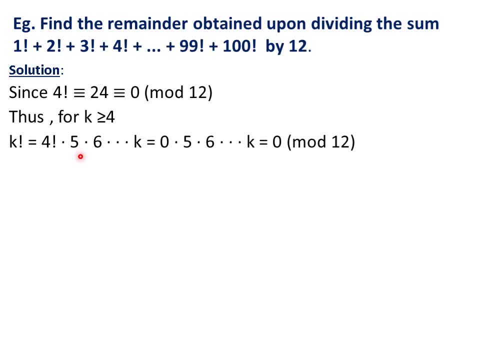 like this, that is, k factorial will be 4 factorial into 5, into 6, up to so on k, But 4 factorial is congruent to 0 mod 12. therefore this whole multiplication is congruent to 0 mod 12, right? So this implies for all the integers which are greater than or equals to 4, their 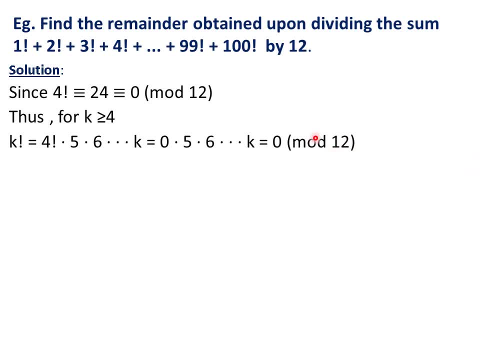 factorial is divisible by 12 because of the factor 4 factorial. okay, So in this sum we can see that 4 factorial, 5 factorial, up to so on 100 factorials. all these numbers are congruent to 0 mod 12.. So only remain is to find the remainder, when 1 factorial plus 2 factorial plus 3 factorial is. 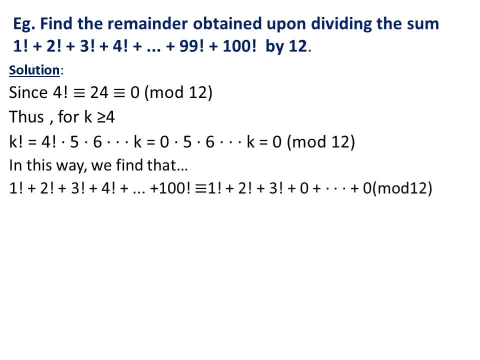 divisible by 12.. So that is, we can write it like this one, this whole equation. so 1 factorial is 1, 2 factorial is 2, 3 factorial is 1.. 4 factorial is 6 and their addition is 9. therefore, 9 is the remainder, which is obtained after dividing. 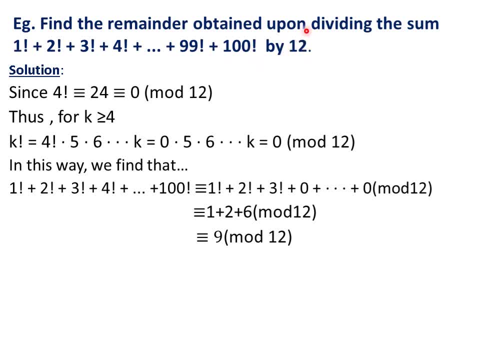 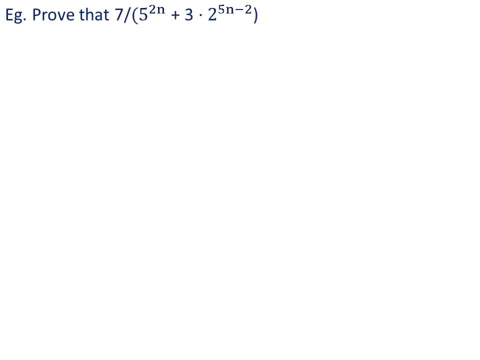 this whole sum by using 12.. So 9 is the answer. So this is one example for practice. you can solve it. In this example we want to prove that 7 divides the sum pi raise to 2, n plus 3 into 2 raise to pi, n minus 2. okay, So to do this, we will find out their respective. 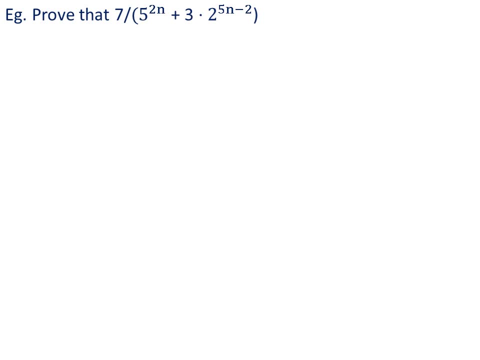 remainders when they are divided by 7, and then finally we will add them together. okay, So let us start with pi raise to 2 n. So for this we know that pi is congruent to minus 2 mod 7. by taking its power as 2 n, we will get it as minus 2 raise to 2 n, but 2 n is even number, so it will be. 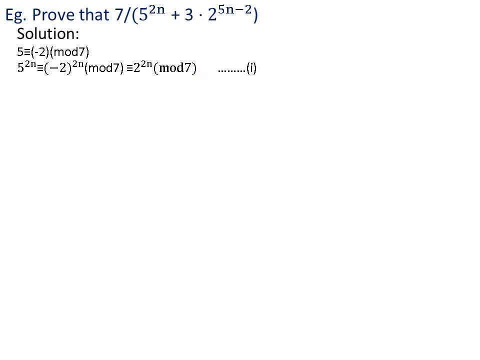 just 2 raise to 2 n mod 7. So let us give it name as 1. okay, Now consider this second term. let us make from adjustment. that means by multiplying and dividing by 2. here we will get this term. 2 into 3 will be 6, and 1 upon 2, that is two inverse. it can be added to this power so that we will get: 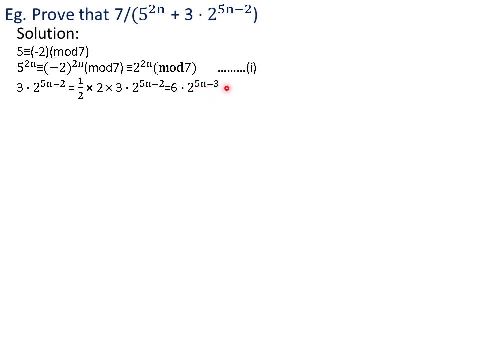 it as 6 into 2, raise to 2? to phi n minus 3. okay, so by taking, by dividing this term by 7, since 6 is congruent to minus 1 mod 7, so it can be written as this right. so by equation number 1 and 2, if we will add: 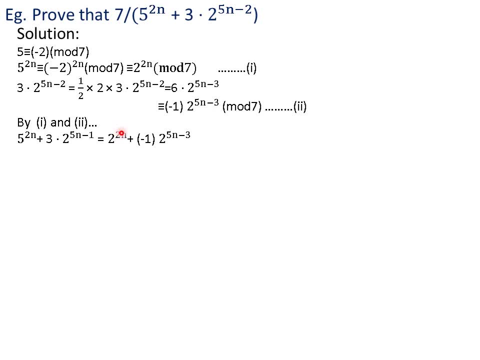 this together, then we will get it as 2 raised to 2n plus minus 1 times 2 raised to phi n minus 3, right? so if we will take 2 raised to 2n common, then in bracket we will get it as 1 minus, as phi n can be written as 2n plus 3n, right? so if we will take 2 raised to 2n.